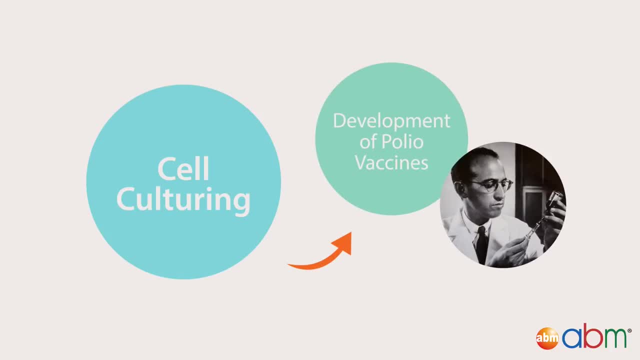 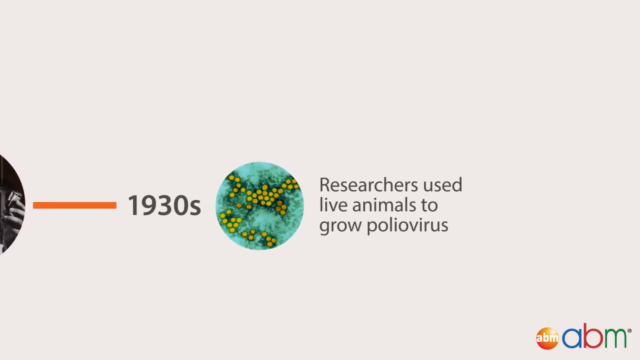 One of the major contributions of cell culturing is the development of polio vaccines. Back in the early 1930s, researchers had to use live animals to grow poliovirus, But with cell culture researchers were able to have greater control of virus production, which 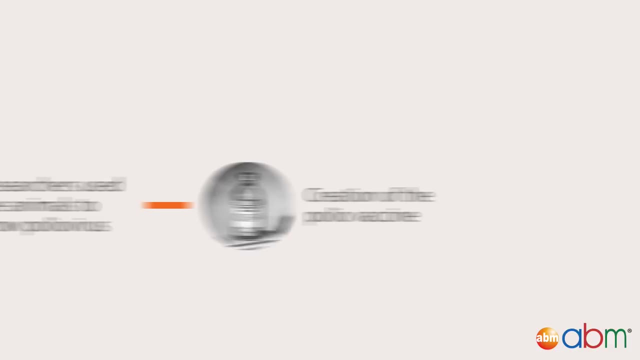 eventually led to the creation of the vaccine. Fast forward to the 1970s, mammalian cell culture was used to create properly folded and glycosylated proteins, such as interferons and antibodies, that were impossible to make in prokaryotic E coli cells. because E coli cells lack post-translational modifications, 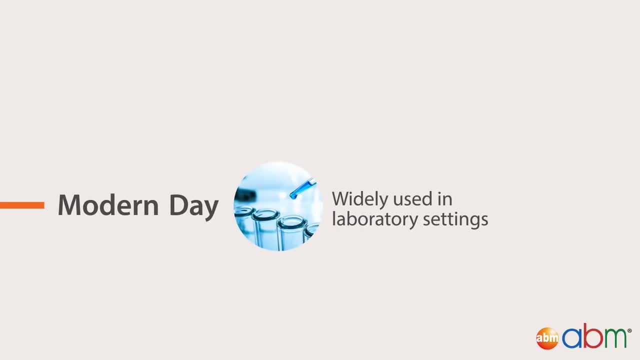 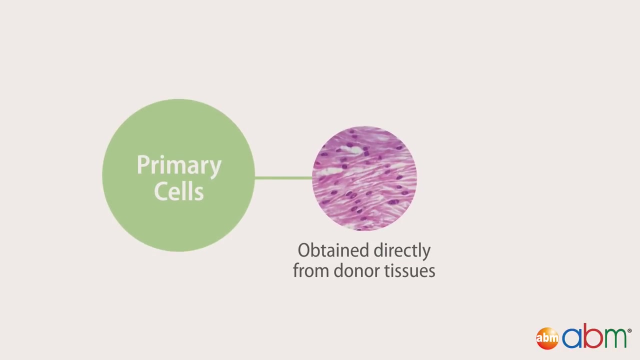 Nowadays, cell culture is being used widely in laboratory settings, particularly in the fields of vaccine research, cancer research and protein therapeutics. Cells that are used in laboratories can be generalized into two categories: primary cells and established cell lines. Primary cells are cells that are directly prepared from 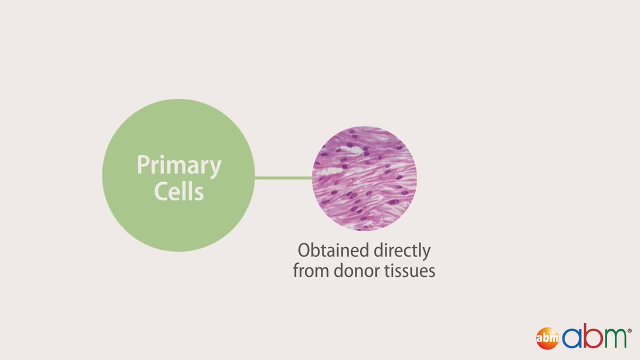 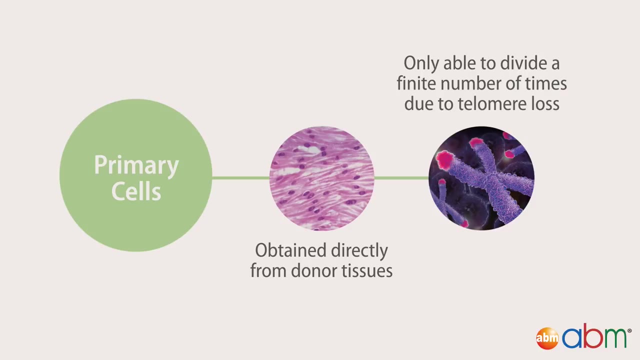 an organism's tissues. If grown under the right conditions, primary cells will grow and proliferate, but they are only able do so a finite number of times. This is because each time as the cells divide, part of its DNA's telomere is lost and 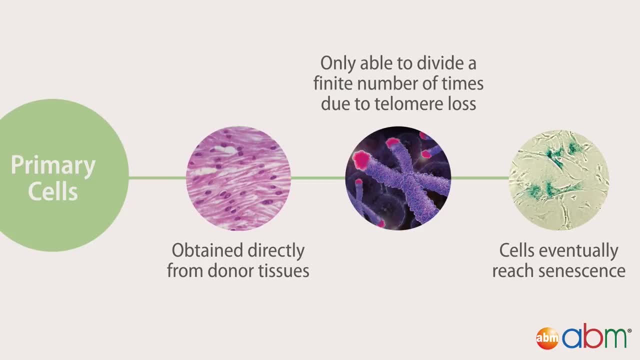 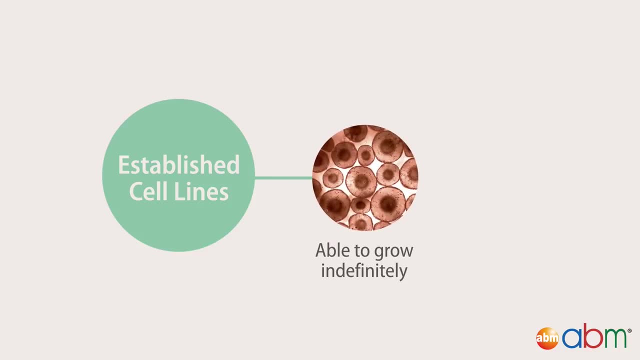 after a certain number of cell divisions, the cells would reach senescence. when the cells can no longer divide, Established cell lines, on the other hand, are able to escape the normal constraints of the cell cycle and grow indefinitely, making them extremely useful for long-term research. 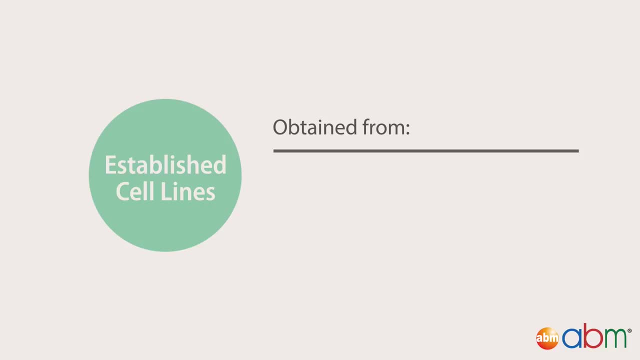 Whereas primary cells are obtained directly from donor tissues, cell lines can be derived from clinical tumours or created from transforming primary cells with viral oncogenes or chemical treatments. These reagents or treatments target one of the checkpoints in the five phases in the 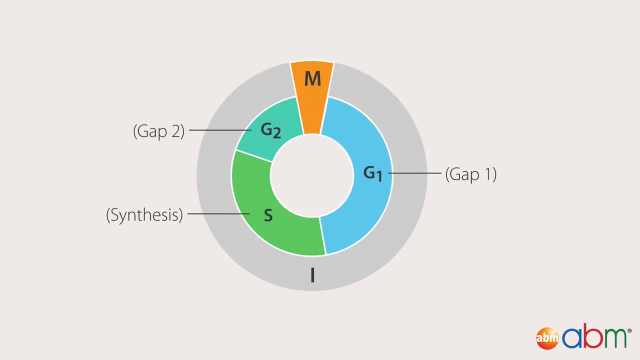 mammalian cell cycle. Checkpoints are there to ensure that the cell meets the appropriate requirements in order to move on to the next stage of making donor cells. One of the checkpoints is at the end of G1,, which allows cells to commit to cell division. 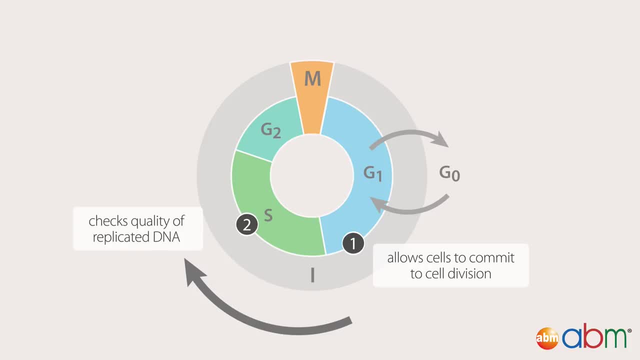 The second checkpoint is at the S-phase and is there to check the quality of the cell. The third checkpoint is after G2, and its purpose is again to ensure that DNA has been replicated completely and is undamaged. Finally, there are several checkpoints within mitosis to ensure that the cell is in a proper 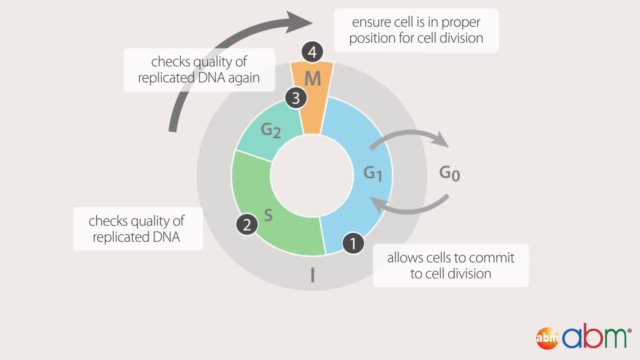 position to complete cell division. When a cell starts to divide uncontrollably, it is because they have evaded these checkpoints and the cell cycle is allowed to proceed. The second checkpoint is at the S-phase and cells continue to proliferate. 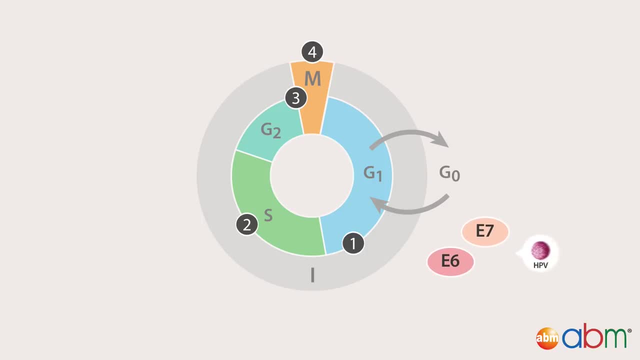 Many viral oncogenes, such as E6 and E7 from the human papillomavirus, can degrade controllers of the cell cycle, namely the tumor suppressor genes, to turn a normal cell. cancerous Primary cells and established cell lines in culture usually adopt one of the two growing 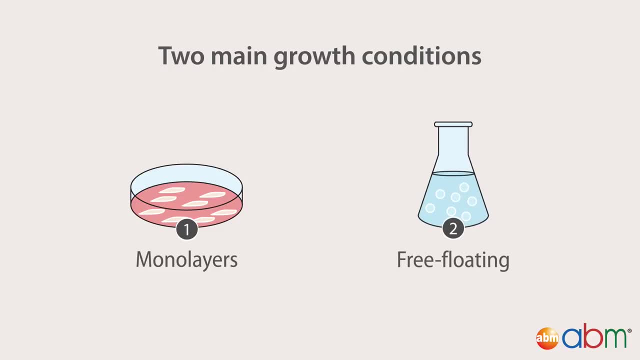 forms. They either grow as monolayers or are free-floating in culture media. Cells that form monolayers are also often referred to as adherin cultures, while the free-floating cells are called suspension cultures. Knowing the growth properties of the cells can help scientists choose the appropriate 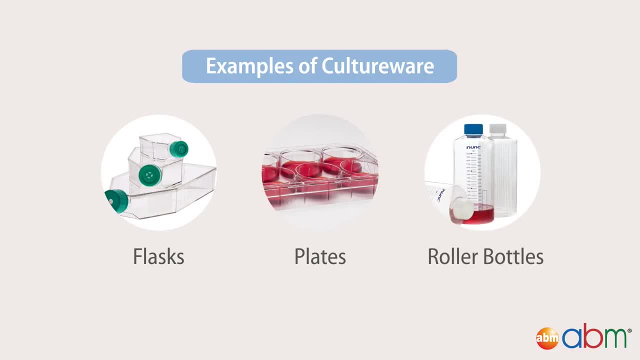 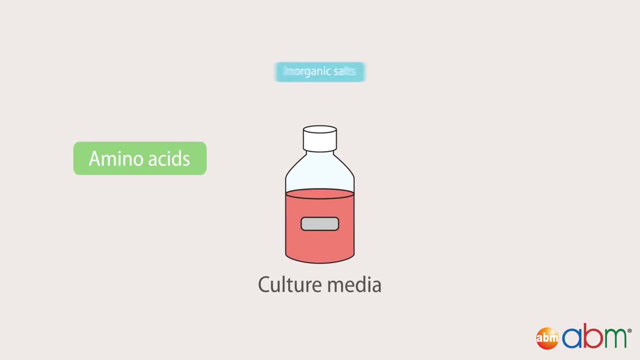 culture wear for their experiments. To keep the cells alive, it is important to keep the conditions as close to the physiological conditions as possible. Therefore, supplements such as amino acids, inorganic salts and vitamins are added into the culture media. The cell is then processed to form monolayer cells. 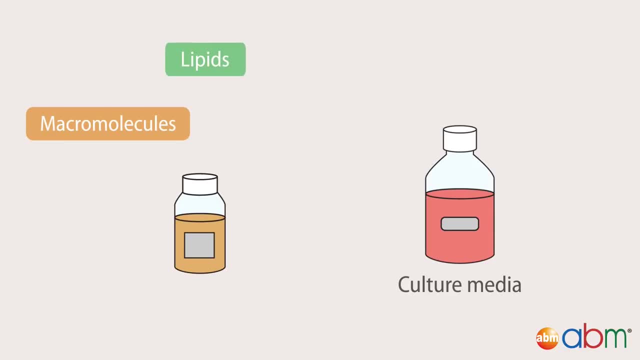 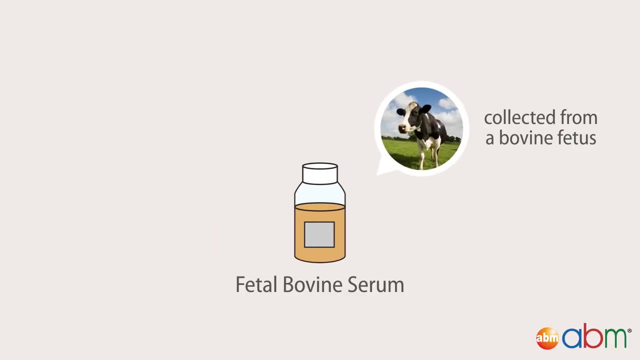 Additionally, other vital supplements, including macromolecules, lipids and growth factors, are supplemented in the form of fetal bovine serum, or FBS. However, there are a lot of uncertainties with regards to the use of FBS, For example, as scientists do not know the serum's exact composition. it is always 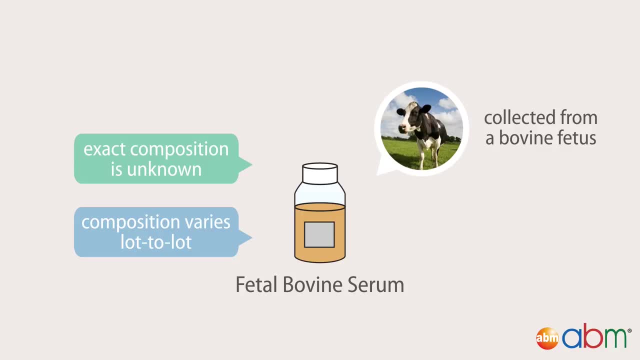 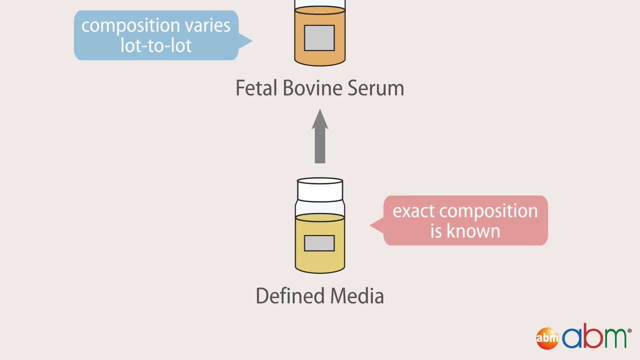 subjected to lot-to-lot variation, and this, in turn, can affect the cultures. Recently defined media, where the exact composition of the media is known, are on the rise to address this issue. As physiological fluids have a neutral pH, the culture media also have a buffering system. 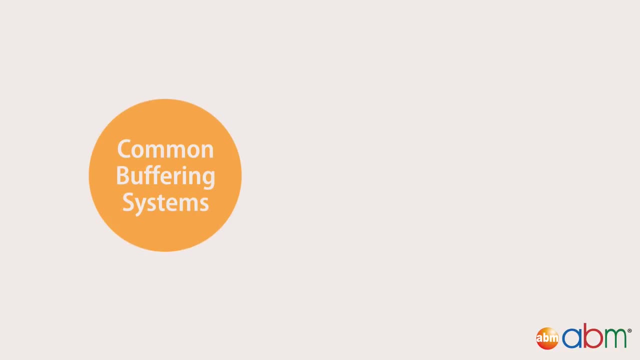 to ensure that the proper pH is maintained. One way to achieve this is to use sodium bicarbonate to keep the pH of the media between 7.2 and 7.4, with 5-10% gaseous carbon dioxide. Another common buffering system involves the use of switter ions such as Hepis. 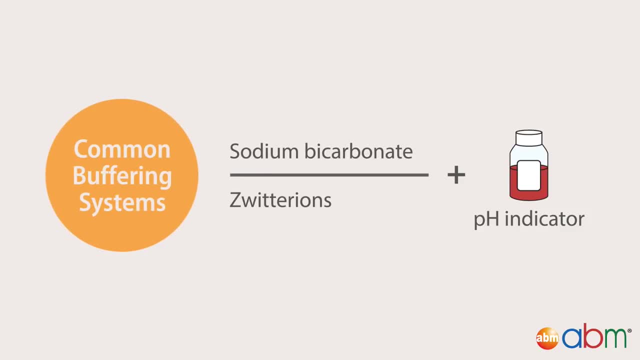 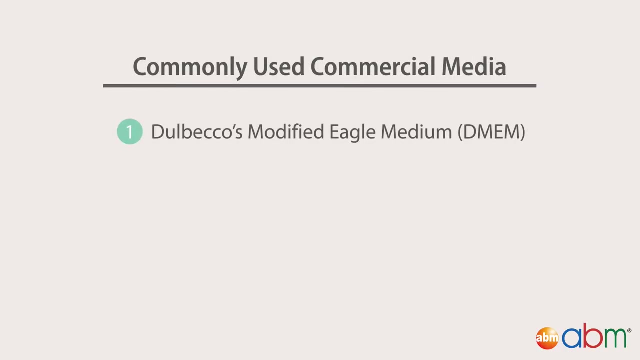 In both kinds it is common to have a pH indicator such as phenol red, added to the media so the cells can visually monitor the changes in pH. Different cell lines generally require different types of media, and the most commonly used commercial media today are Delbecco, Modified Eagle Medium. Roswell Park Memorial. 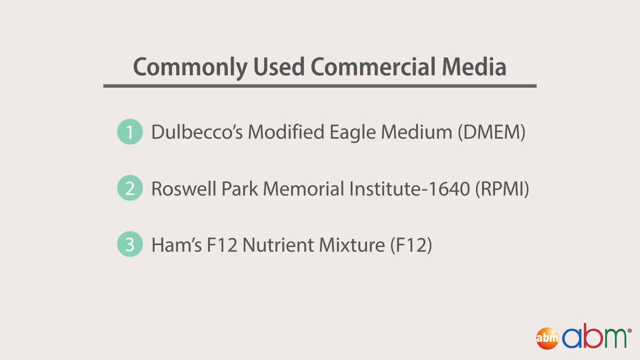 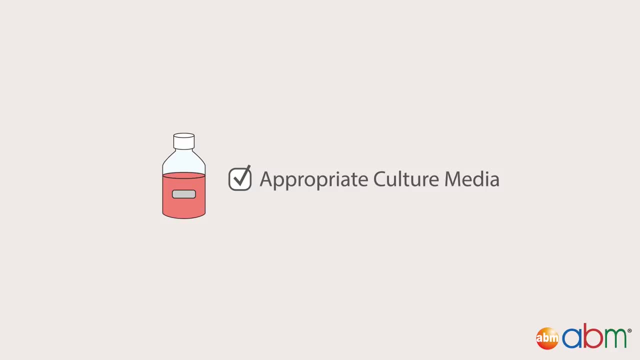 Institute 1640 and Ham's F-12 nutrient mixture. Apart from using the appropriate media for growth, the cells are also maintained in the correct temperature. For example, most mammalian cells are incubated at 37°C for optimal growth, while cells derived. 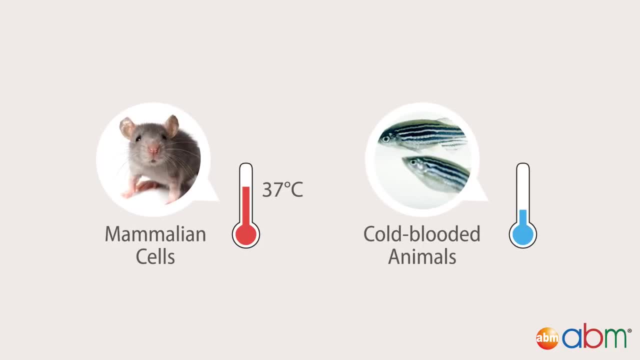 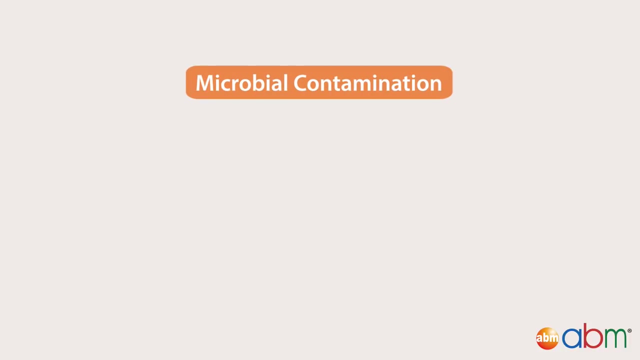 from cold-blooded animals should be kept at lower temperatures. Other measures to take when working with cell cultures is to ensure that the cells are kept under a sterile environment. Microbial contaminants such as bacteria, fungi or mycoplasma can ruin the culture and lead. 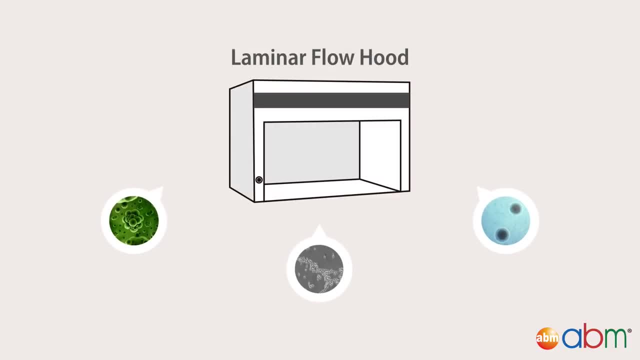 to invalid experimental data. A laminar flow hood is always used for cell culture work. It maintains a steady, clean airflow and prevents outside contaminants from entering the culture. In addition to microbial contaminations, the cells can also be contaminated by other cells. 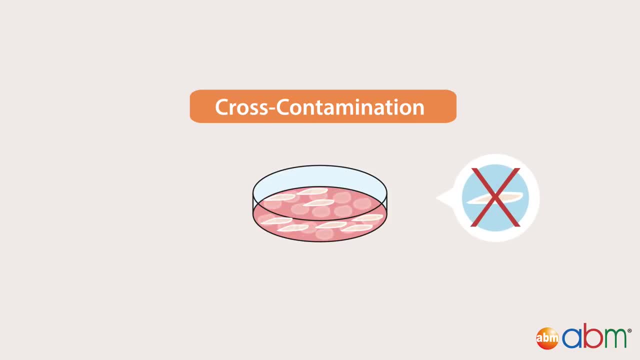 Cell lines can be overgrown and replaced by other fast-growing cells inadvertently introduced into the original culture. The consequence of using a misidentified cell line is making false scientific conclusions. Authenticating cell lines using short tandem-repeat processes can be very difficult. In addition, cell lines can be overgrown and replaced by other fast-growing cells inadvertently. 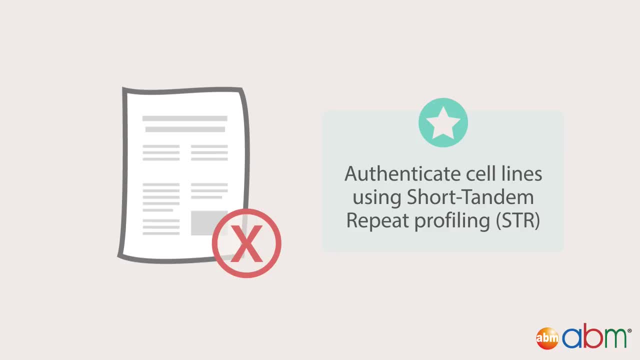 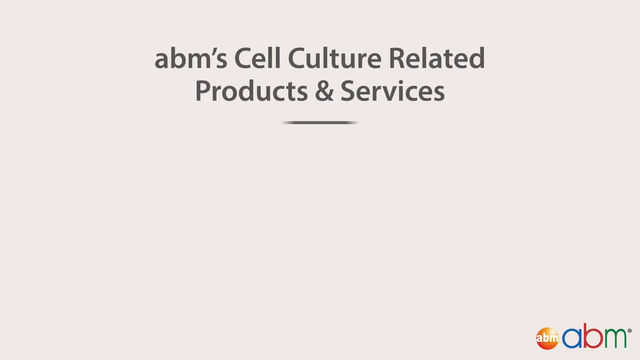 introduced into the original culture. Cell line profiling, or SDR, is recommended for cultures from time to time. ABM provides a wide range of cell culture-related products, ranging from the starting materials, such as primary and immortalized primary cells, to immortalizing agents, media and plastic. 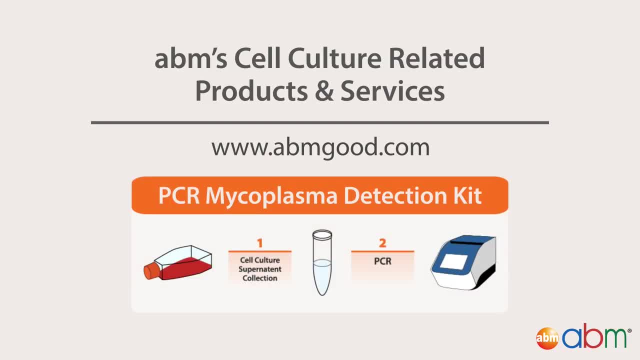 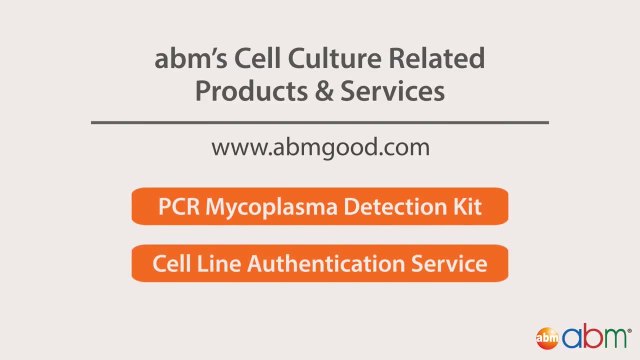 wear. We also have specialized PCR-based detection kits and drug treatments for mycoplasma contamination. Lastly, since many scientific journals and funding agencies now require evidence of cell line authentication by SDR profiling as a record, we have a wide range of cell culture-related 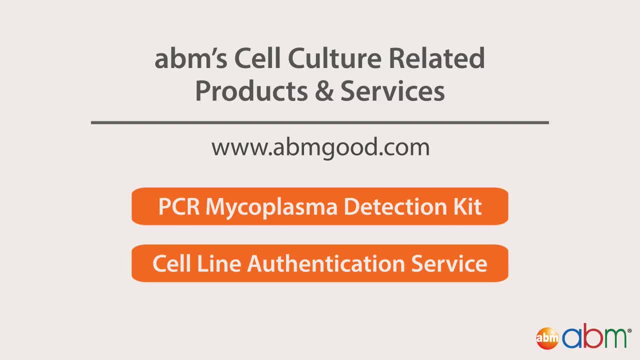 products ranging from the starting materials, such as primary and immortalized primary cells, to immortalized primary cells. We are proud to now offer this service to our customers. Cell Culture Technique has advanced our scientific knowledge since the 1930s and it continues to provide us valuable information about all aspects of biology. If you'd like to read more, please visit our Knowledge Base at the link below. Also, be sure to check out our next video for Cell Culture Techniques. Please leave your questions and comments below and we will answer them as soon as we can. 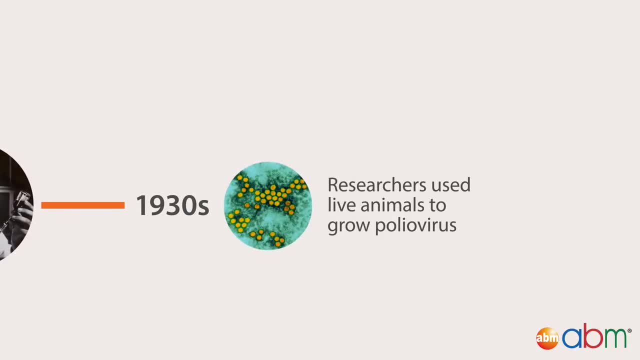 Thank you for watching this video. We hope you enjoyed it. If you liked it, please subscribe to our channel. If you want to learn more about cell culture techniques, please check out our website at wwwcellculturetechniquecom. If you have any questions or comments, please leave them in the comments below. 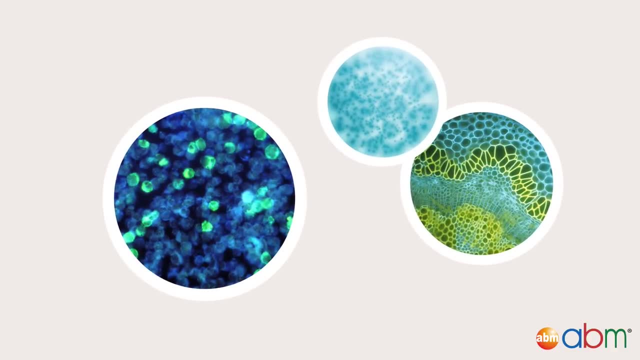 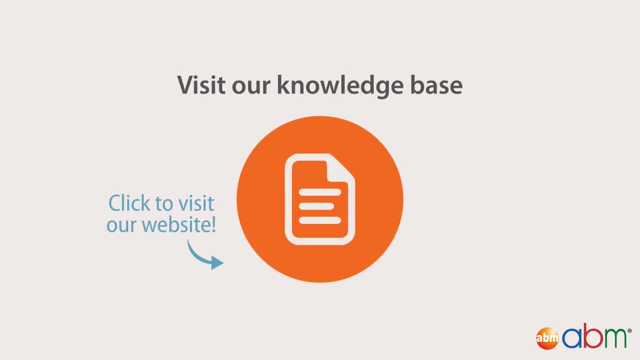 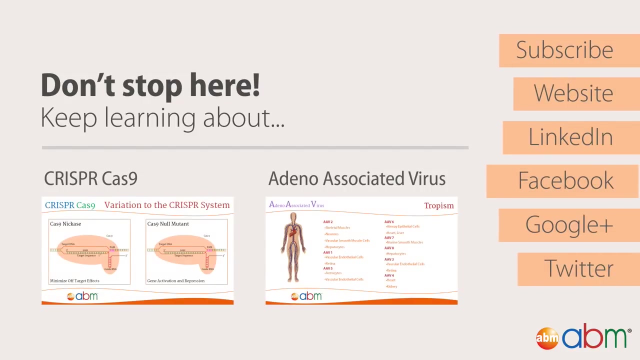